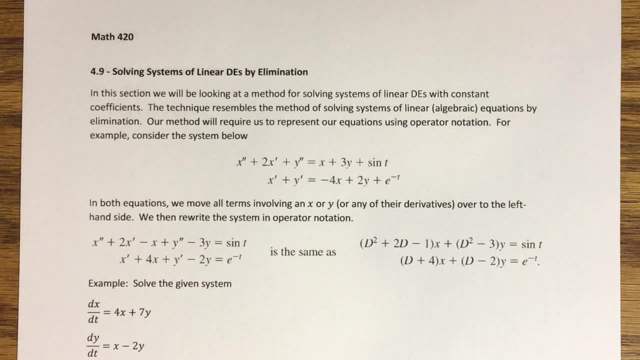 and we will explore it in much more depth in a later chapter- It's going to be towards the end of this course. we look at these systems in more depth, But this is one technique that we could use to solve these linear DEs and it mimics what you do when solving different systems of equations in algebra. 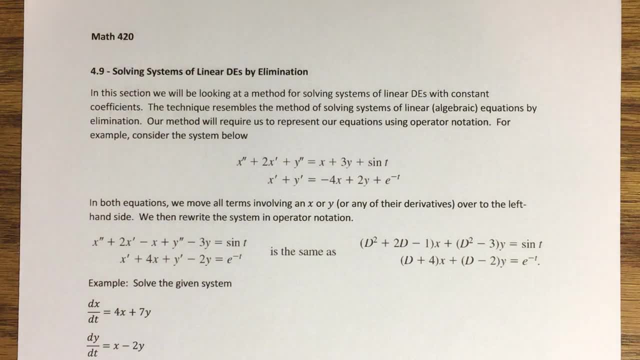 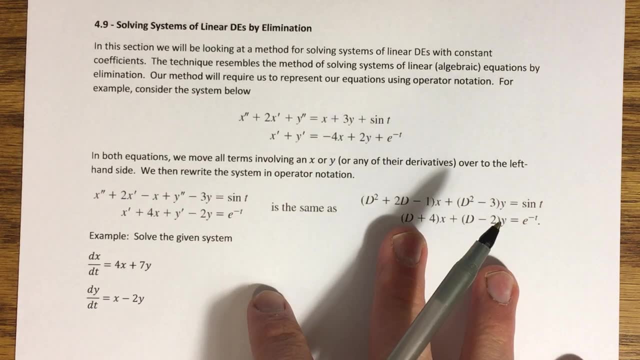 using a technique by the same name: elimination. So before we get into that, we're going to talk about how we're going to represent our differential, our systems of equations before solving them. Here's an example of a system of two differential equations: linear differential equations. 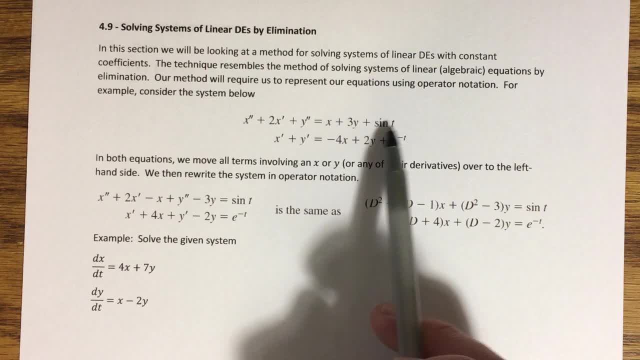 X and Y in these equations are thought of as functions of T. So the first thing you want to do is get all of your X's and Y's, as well as all of their derivatives, second derivatives and so on, all over to the left-hand side and then get any functions of T to the right-hand side of both equations. 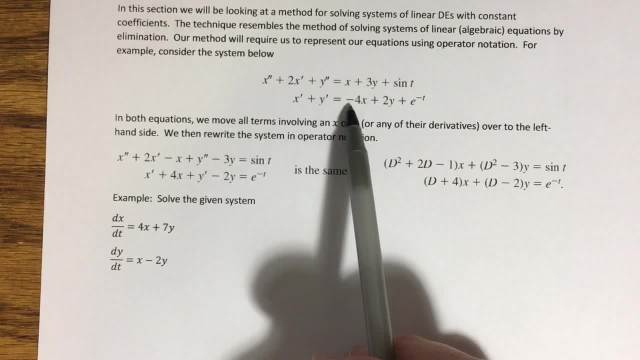 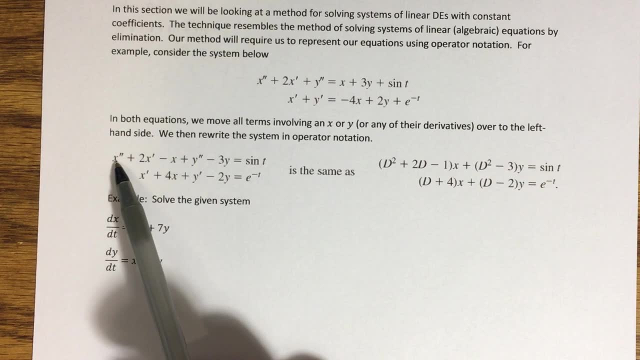 So that's what's going on here. We've taken anything involving an X or a Y or any of their derivatives, move them over to the left, and that's what you're seeing here. I'm also being careful to keep all of the X's together and all of the Y's together, like this. 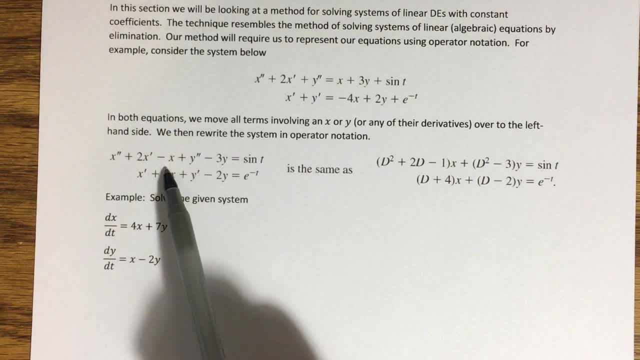 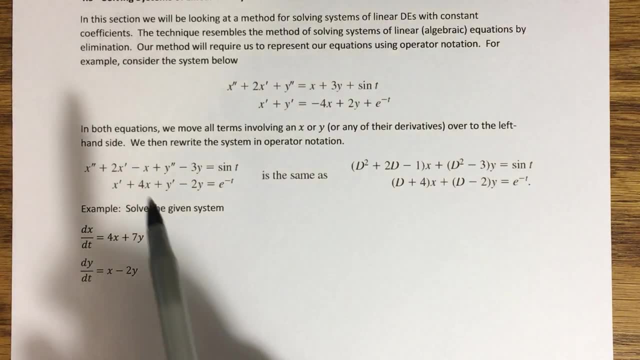 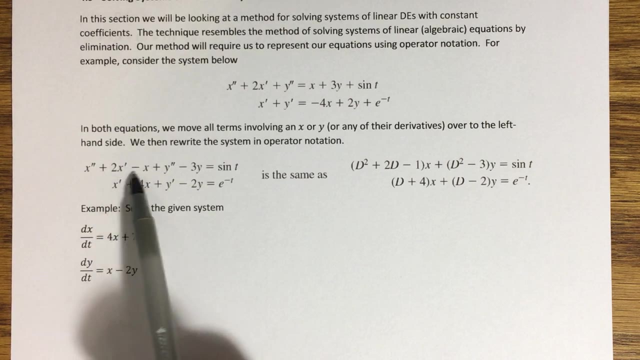 Okay, next thing I want to do is rewrite the left-hand side of each of these equations in operator notation. So, remembering operator notation, I have X, double prime plus 2x, prime minus X here. These 3 X's, and you know X's, with their derivatives, can be written in operator notation this way. 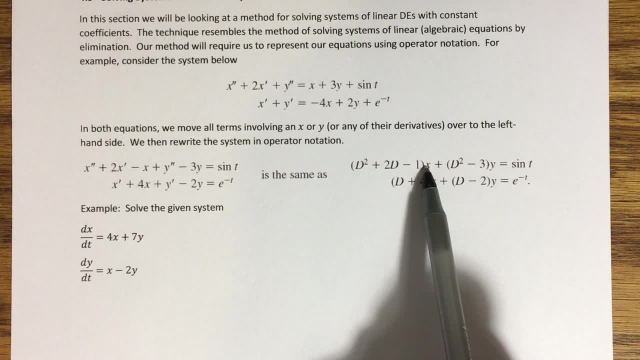 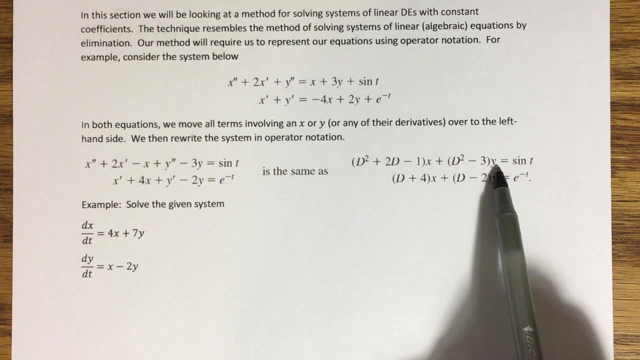 D squared plus 2D minus 1 X. Okay, Same thing as this, just an operator notation. Y double prime minus 3Y is the same thing as D squared minus 3 operating on Y in the. the sine of t is just sine of t. And then I did something similar down in the second part, right? 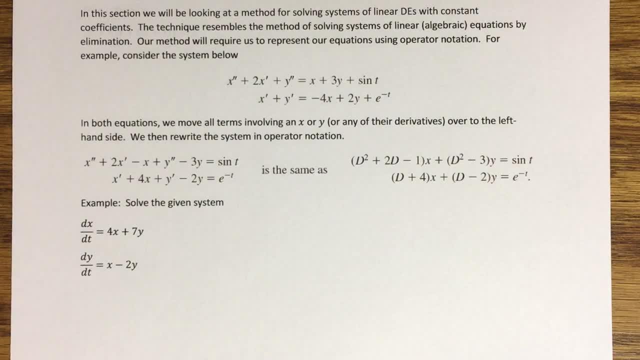 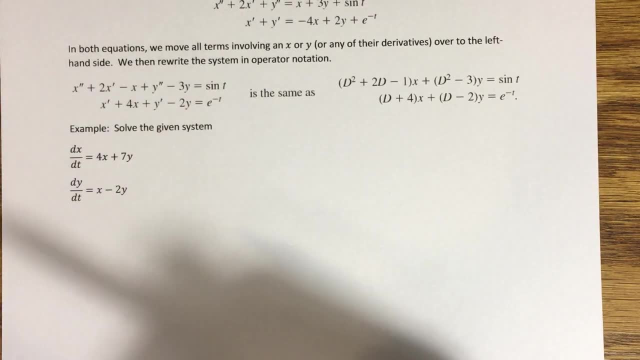 here. Okay, we need our equations to be in that operator form to do what we're going to do when solving these systems, And I'm not going to walk through a general format or technique or derivation or anything like that for solving using elimination. It's best to see how it's done just by. 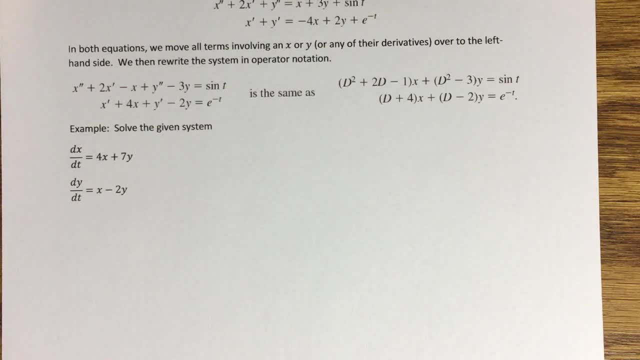 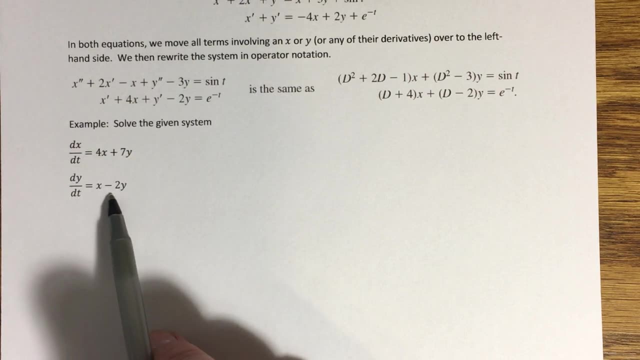 looking at examples, And we're only going to look at two examples in this section. Okay, so let's start with this one. right here I have this system: dx dt equals 4x plus 7y. dy dt equals x minus 2y. All I have are x's and y's and their derivatives, So everything gets moved over to the. 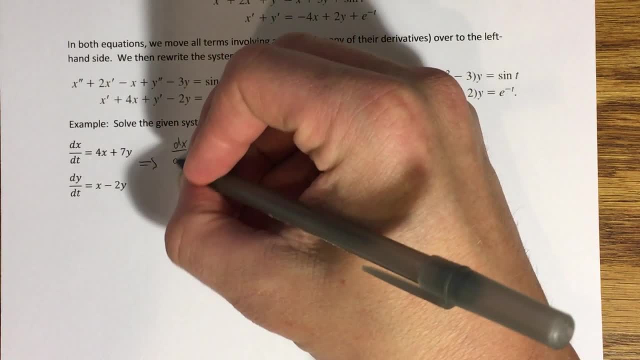 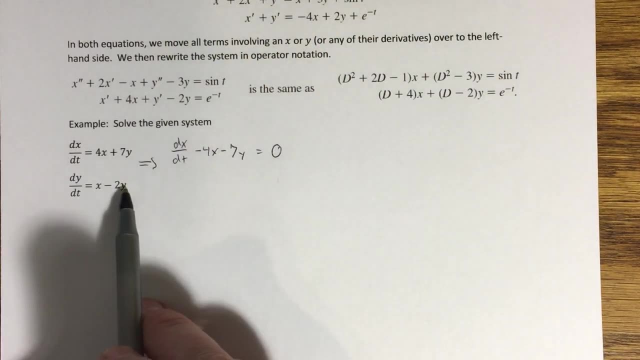 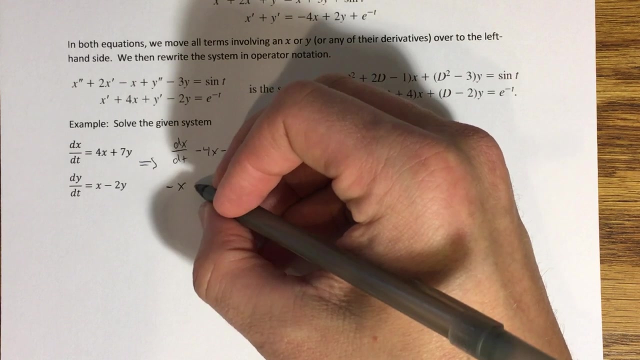 left in both equations. This becomes dx. dt minus 4x minus 7y equals zero. Here I'm going to move everything over and I'm going to make sure that my x terms appear first, So that x gets subtracted over and gives me a negative x, And then I'm going to have a plus. 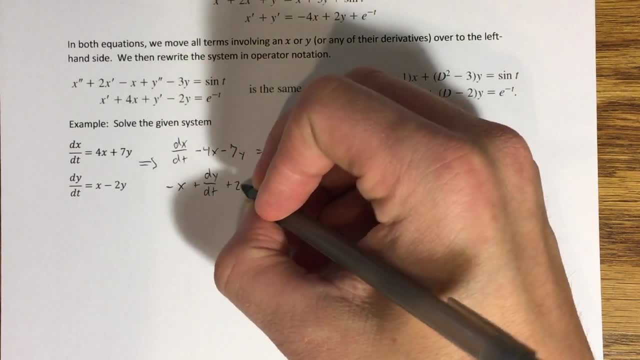 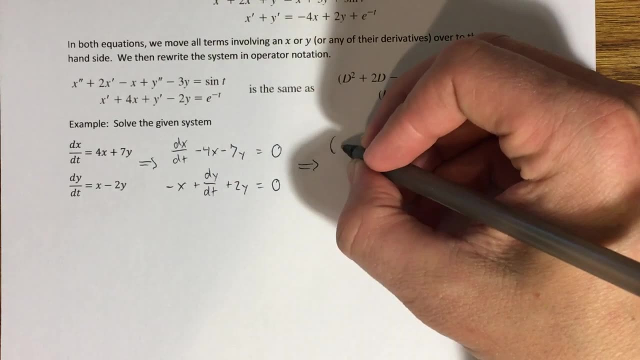 x minus 7y, And then I'm going to have a minus x minus 7y, And then I'm going to have a plus dy. dt plus 2y equals zero. Okay, now, in operator notation this is the same thing as d minus 4x. 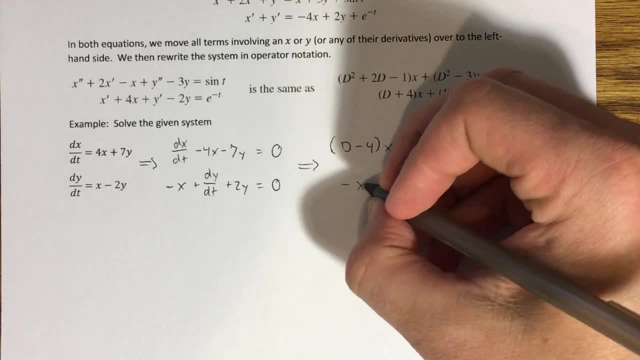 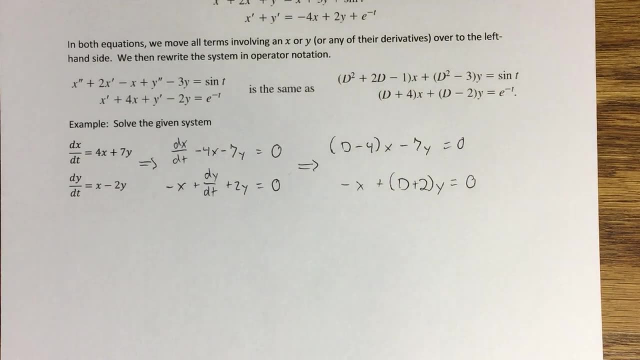 minus 7y equals zero and negative x plus d plus 2y equals zero. Okay, Now here's where we start to use this elimination technique, Once I've gotten this into operator notation- notation the way that I have, If you remember, from algebra, when you want to solve a system of 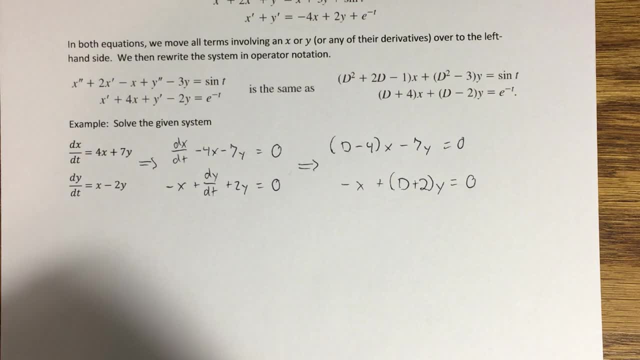 equations using elimination. the goal, as the name implies, is to eliminate one of the variables in that system of equations, And you do that by taking your two equations and trying to get a common coefficient. Or actually, the way I do it is, I get coefficients that are opposites of each. 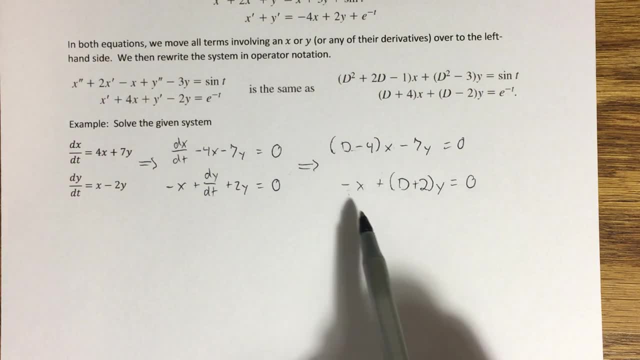 other. So here I have a d minus 4x. I would like for this guy to have a negative d minus 4x, because then what's going to happen is, if I add these two equations, those guys will cancel each other out, leaving me with just y's to worry about. So in algebra, what you're doing is you're. 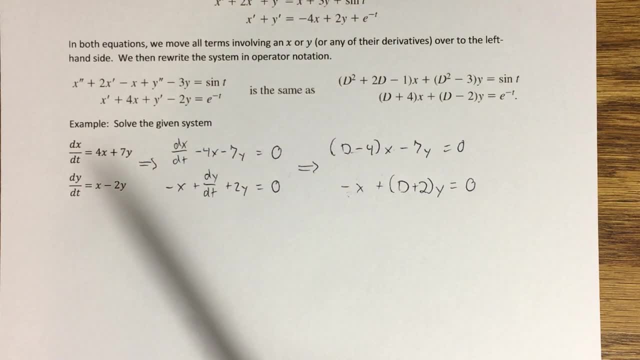 multiplying both sides of an equation by a number. to do that In differential equations, we're operating on both sides of an equation using a differential operator, But differential operators, as we've seen, obey a lot of the same properties as multiplication, In fact. 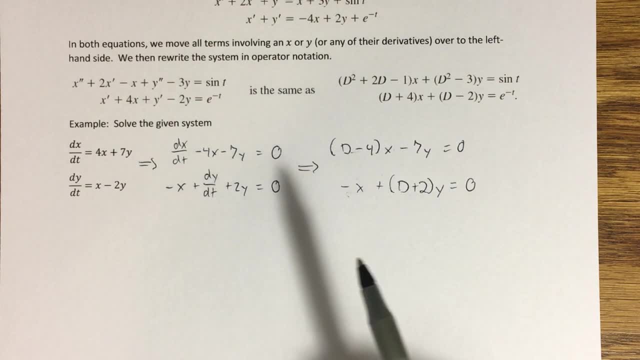 for the purpose of working with them. you can just think of it as multiplication when you're simplifying and doing that kind of stuff. So what I'm going to do is operate on both sides of this equation right here, the second equation- by d minus 4.. So that 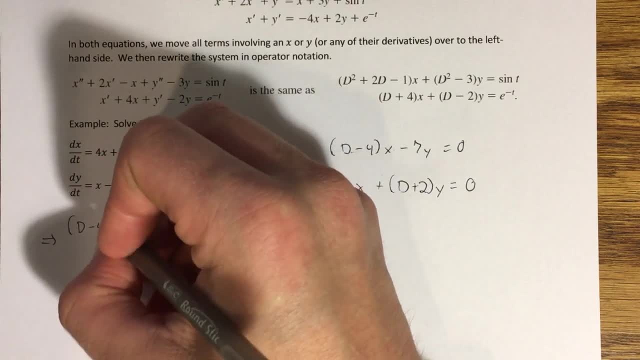 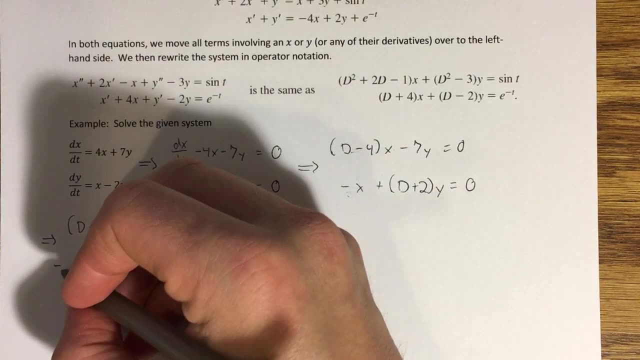 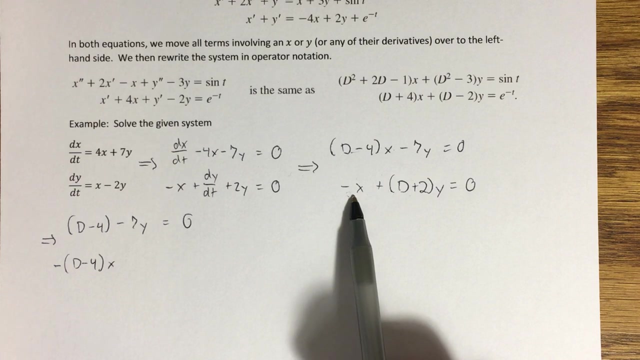 gives me this: My top equation is still: d minus 4. minus 7y equals 0. My bottom equation becomes negative: d minus 4x. Notice, I just operated on this by d minus 4.. And then the negative again, because it kind of works. 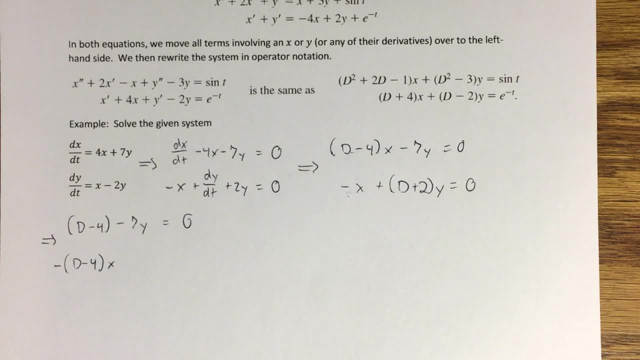 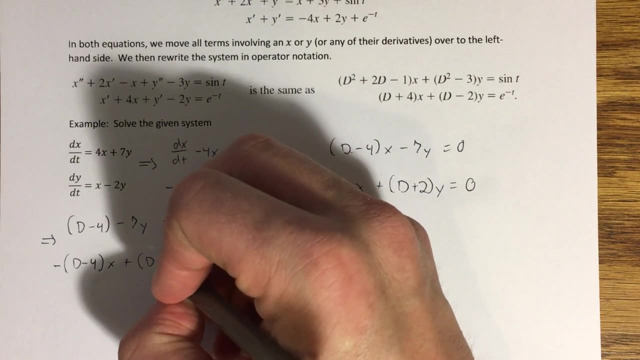 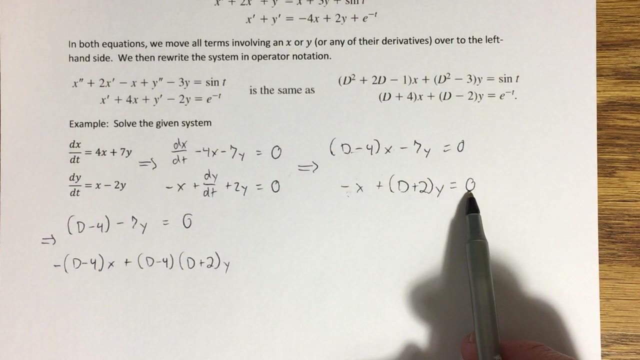 the same way as multiplication. I can think of that as a negative 1, which can come out to the front Plus. this second term is being operated on by a d minus 4 as well, So it becomes d minus 4, d plus 2y, And then here 0. Remember, any differential operator applied to a 0 is still. 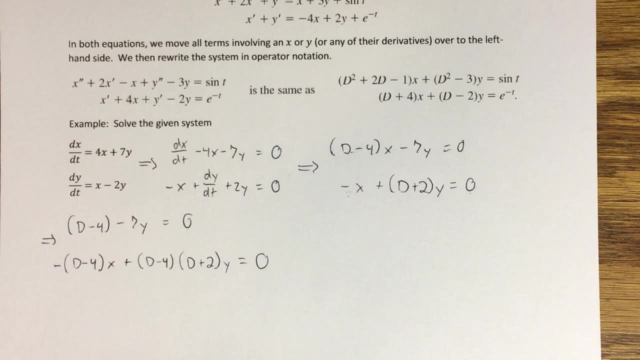 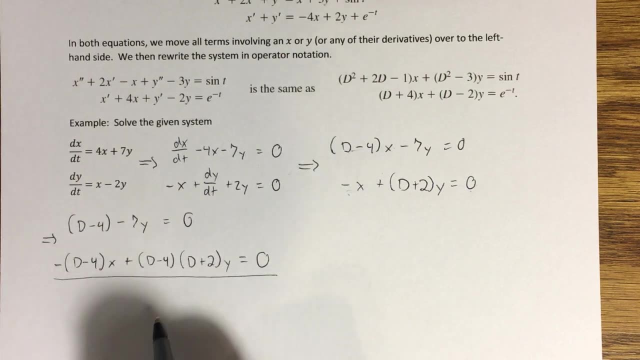 just 0, because 0 is its own derivative and all, So that second equation becomes this: Now, what I'll do is add these two equations. I forgot my x there And you notice I get a cancellation with these two x terms, leaving me with the following: 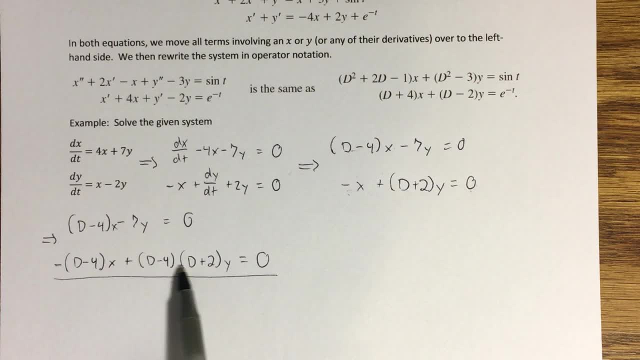 Now this guy right here. I'm going to expand this out. And again you get to think of this composition of differential operators as multiplication. You can actually foil this thing, even though it's technically not the same thing. So I'm going to expand this out. 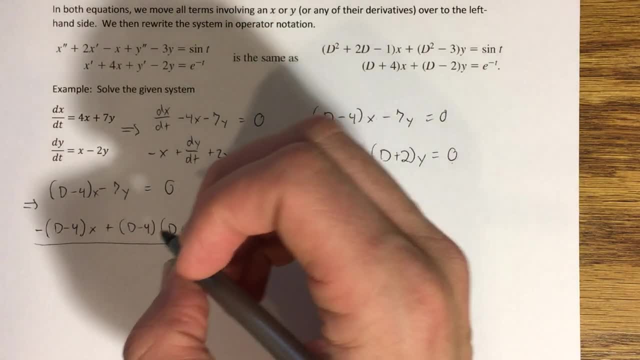 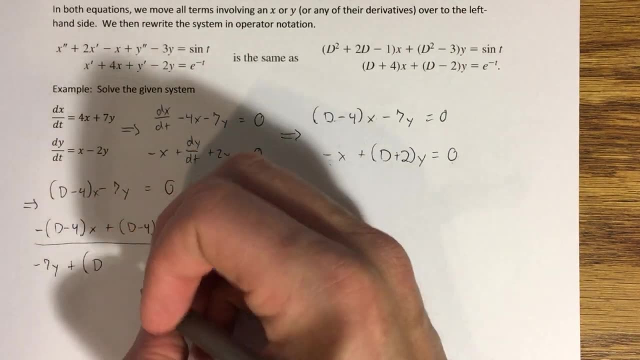 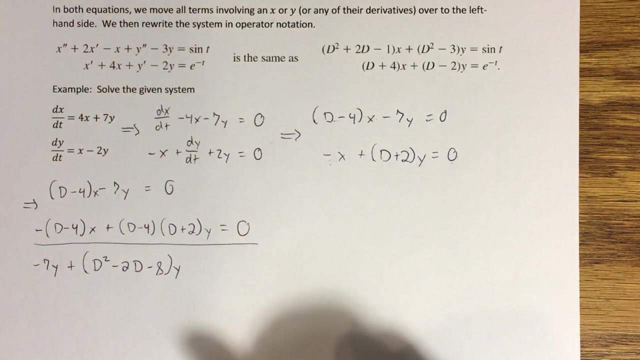 Same thing as multiplication. It still works. So what I'm left with now is negative 7y plus. this becomes d squared minus 2d minus 8y, Okay, And that's equal to 0.. Now what you could do is: 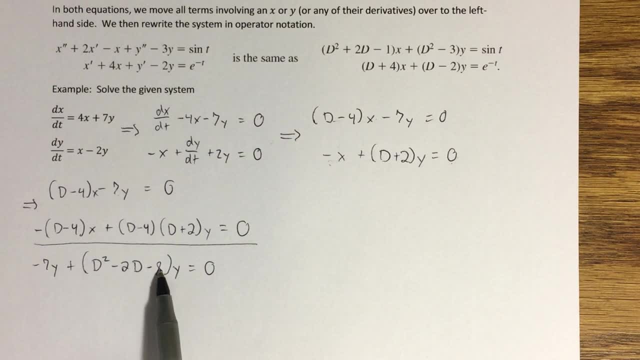 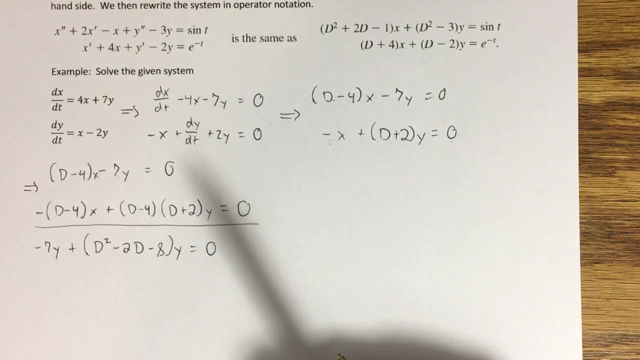 bring the y in to each of these individual operators in parentheses here And you notice one of the things I'll get is a negative 8y And I also have this negative 7y. Those are like terms. You can combine those And they would. 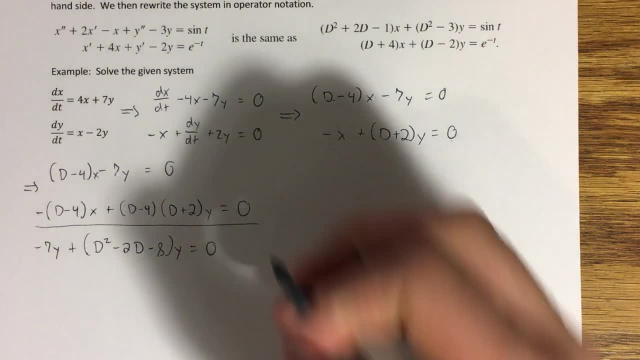 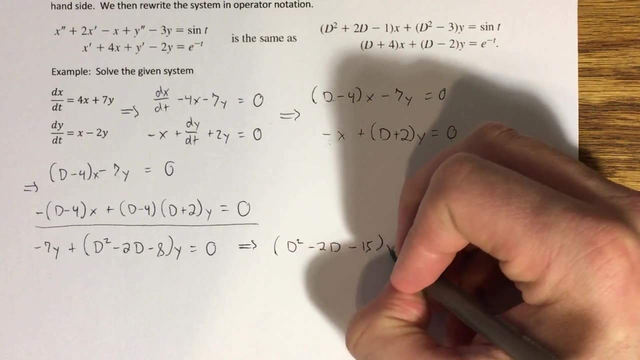 give you negative 15y. So let me actually just change the way that this looks. I'm going to write that as d squared minus 2d minus 15y equals 0.. That's fair enough. I can do that right. 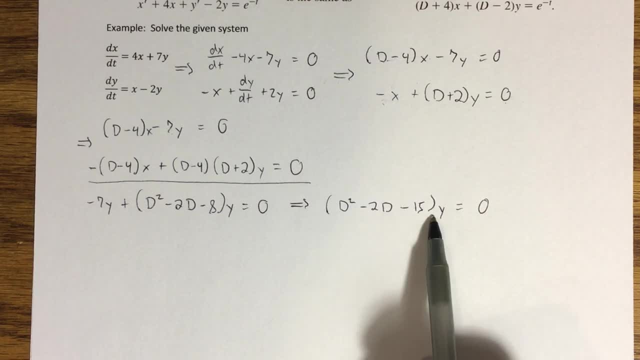 What is this, though? This is a second order linear differential equation. It's homogeneous and it has constant coefficients. This is something that I know how to solve using the techniques that we talked about back in 4.3. And so I'm going to do that. I'm going to solve this thing using those. 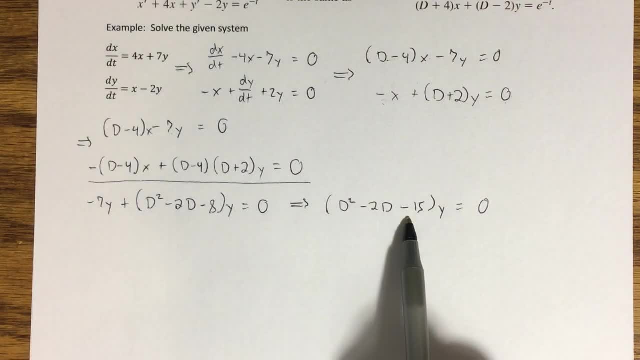 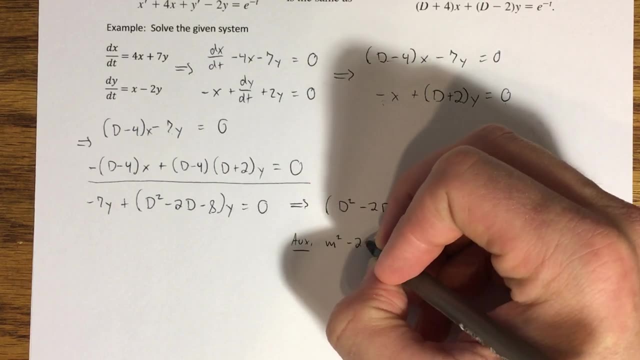 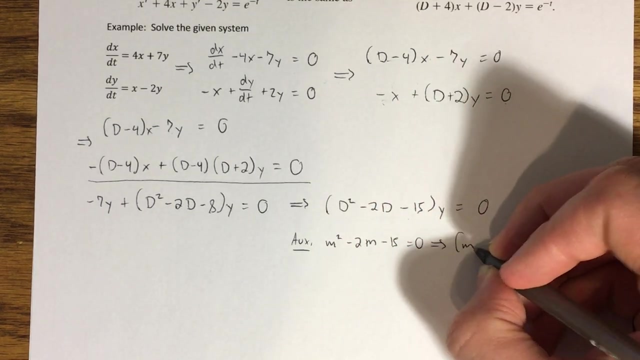 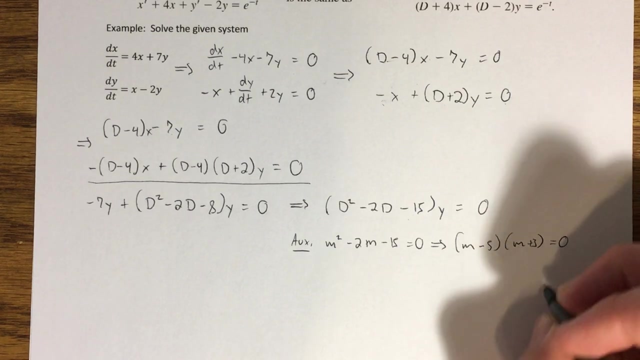 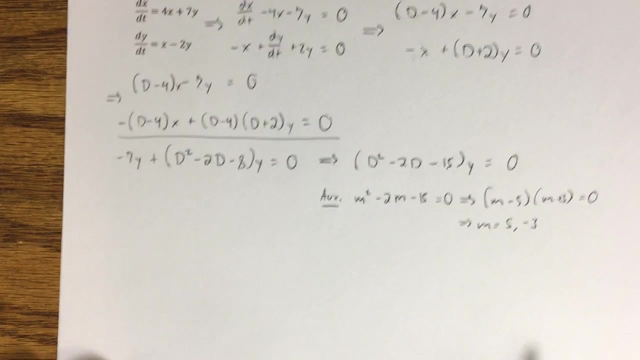 techniques- Notice, because it's an operator notation- I have the form of my auxiliary equation. right away: m squared minus 2m minus 15 equals 0. This thing factors to m minus 5 times m. m plus 3 equals 0, which gives me m equals 5 or negative 3, OK, So right away I have. 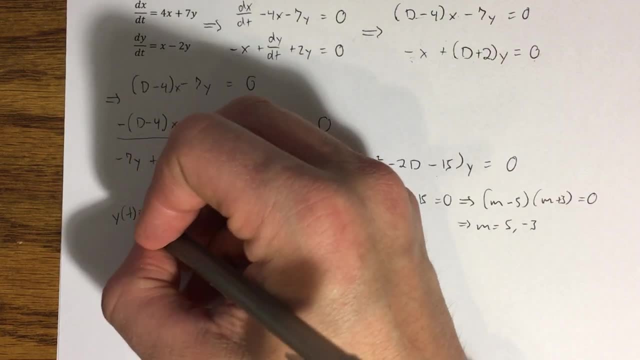 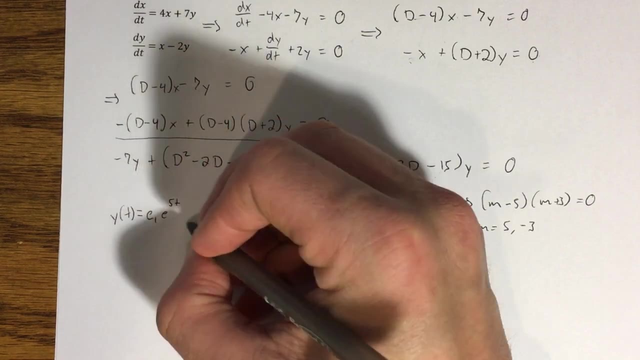 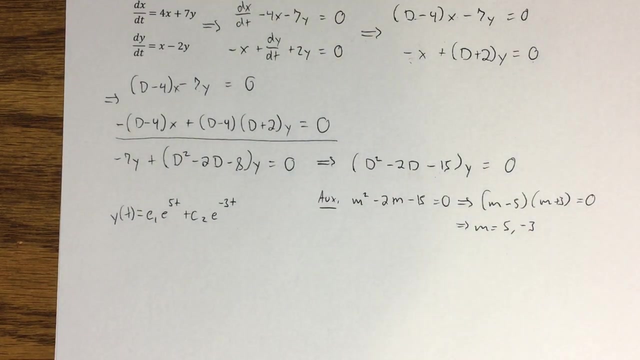 a solution for y. now, y of t is equal to what c1 e to the 5t, plus c2 e to the negative 3t. But it's important to remember that we are talking about a linear differential equation, So I'm going to write that as d squared minus. 5 times m. So I'm going to write that as d squared minus 5t plus c2, e to the negative 3t plus 5t. What I'm going to do is I'm going to write this in the same way that I'm going to write: 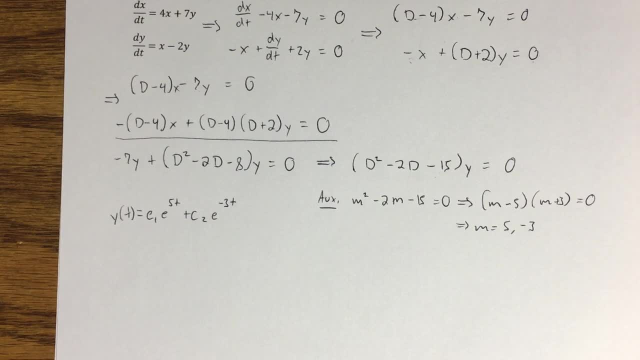 the equation. So I'm going to write that as d squared minus m, and I'm going to write this in the same way that I'm going to write the equation. So now I've got a solution for x, which means that we only have two functions that we're solving. for x and y. I've only 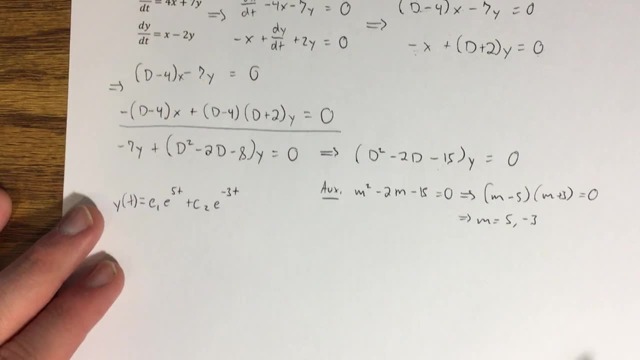 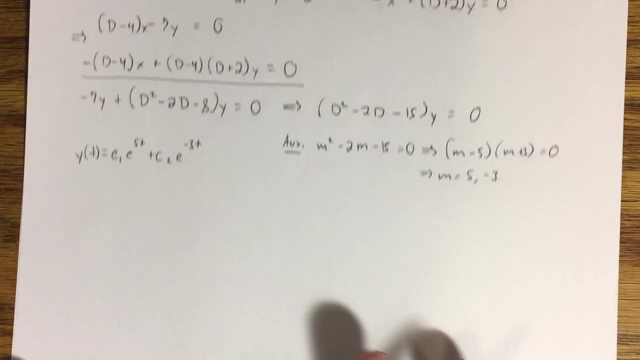 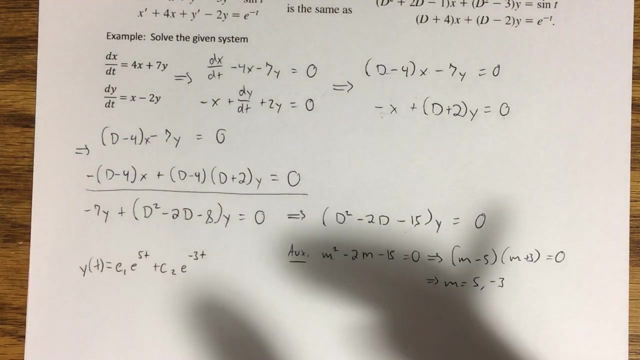 got one solution, So now I need a solution for x. And what I'm going to do? instead of just taking my answer here and substituting it in for y, like you kind of would normally do with a system of equations in algebra, I'm actually going to do elimination. a second. 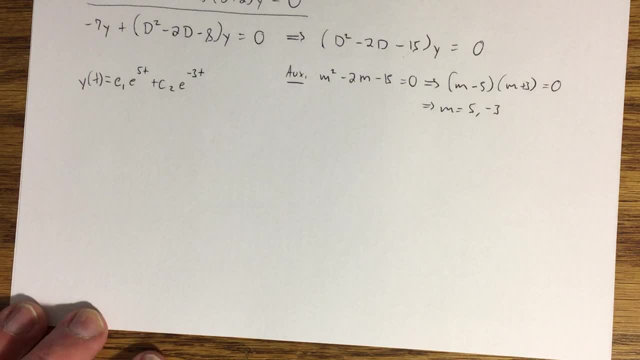 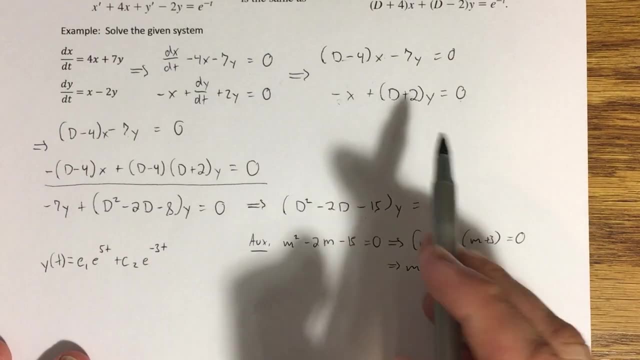 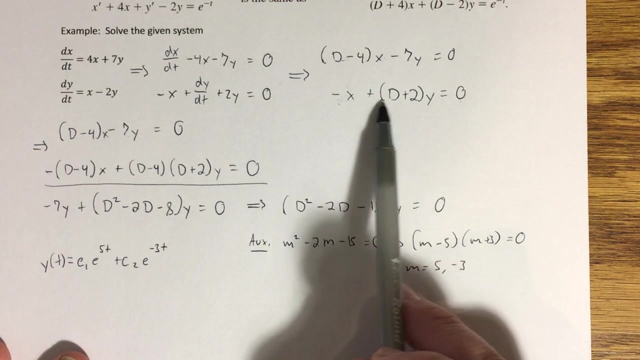 time, but this time intentionally- eliminate the y's, because I'm going to eliminate the the y's, leaving x's left over. Okay, so let's take my system of equations again up here, and my goal now is to eliminate the y term. So notice, I have a d plus 2 showing up here and a negative 7. 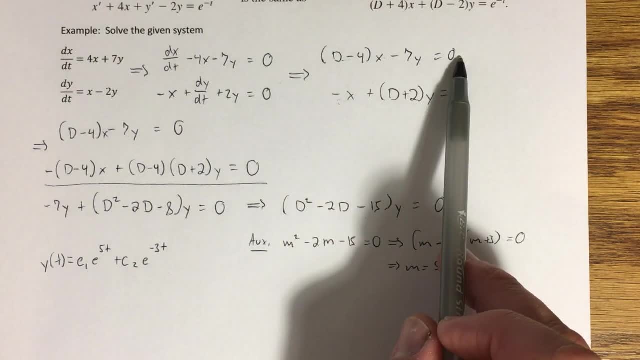 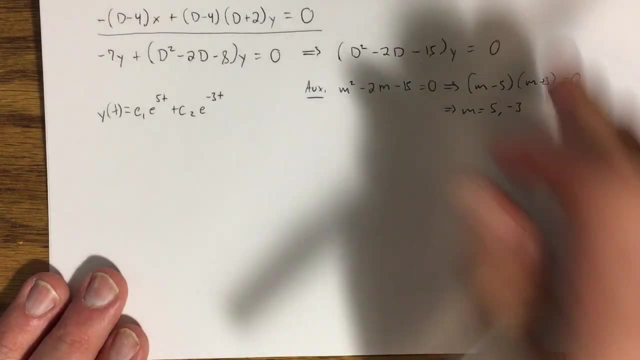 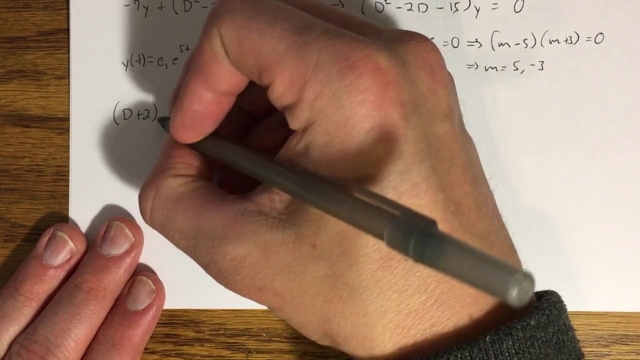 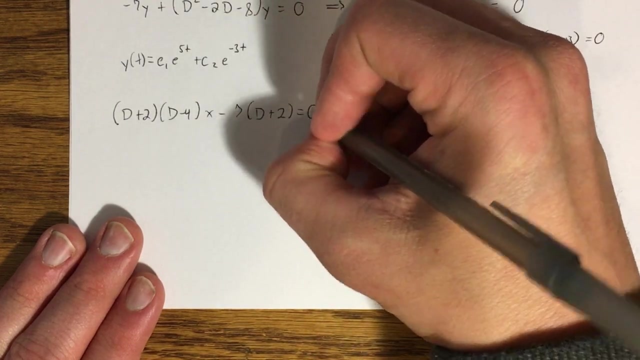 showing up here. What I'm going to do is operate on the top equation by d plus 2 and the bottom equation, I'm going to multiply everything by 7.. So what does that look like? That's going to look like this: d plus 2, d minus 4, x minus 7, d plus 2 equals 0, and then multiplying everything on. 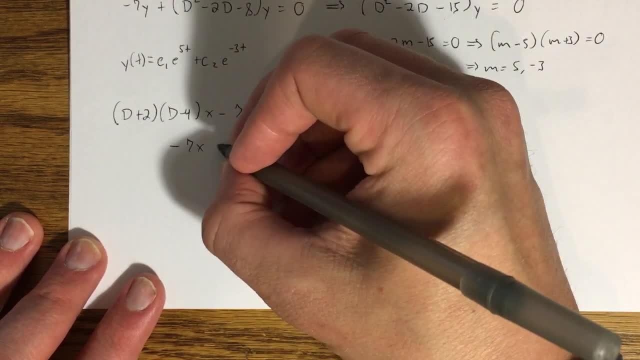 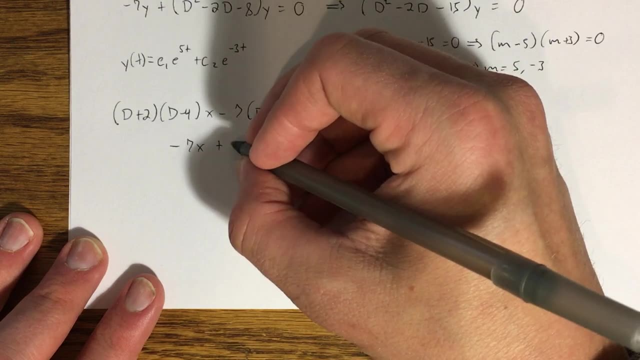 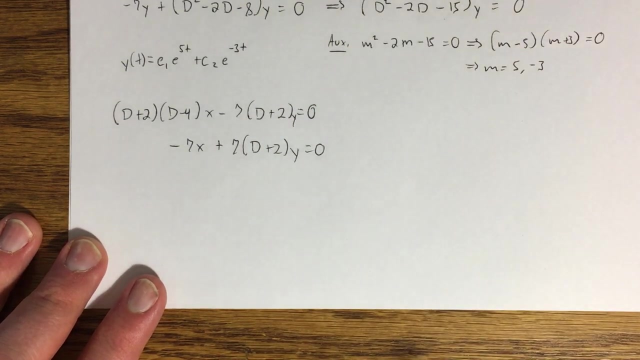 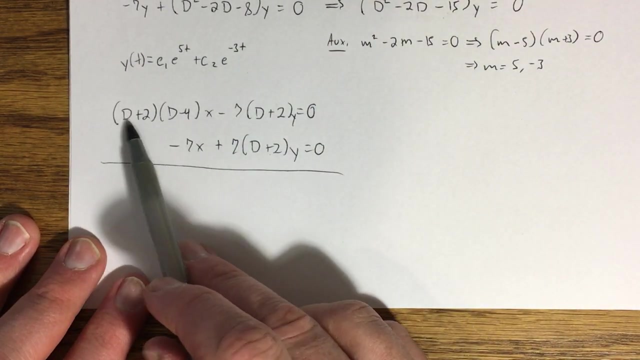 the bottom by 7, I get negative 7. x plus, yeah, positive 7. I'm multiplying by plus 7 times d plus 2y. I forgot my y. there Equals 0. That's going to cause these two terms to eliminate when I add them together. okay, And we're going to. 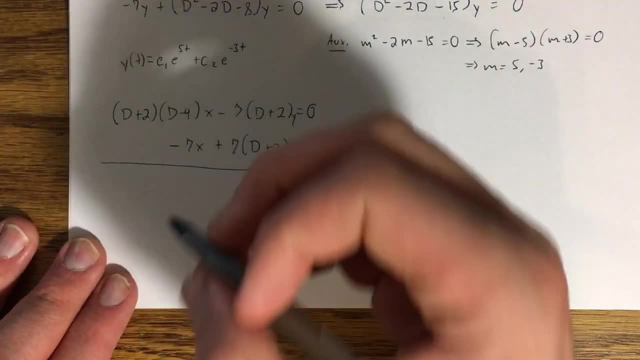 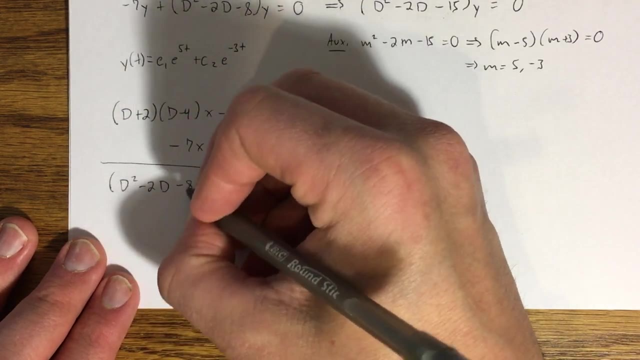 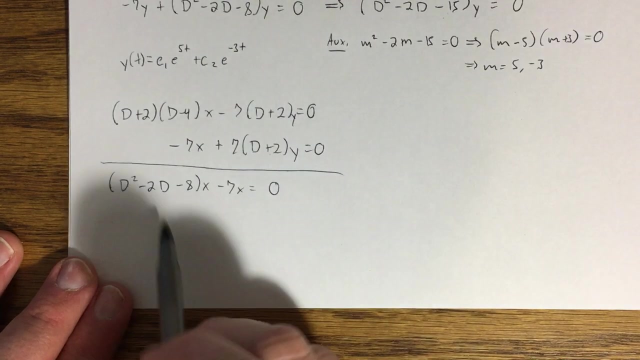 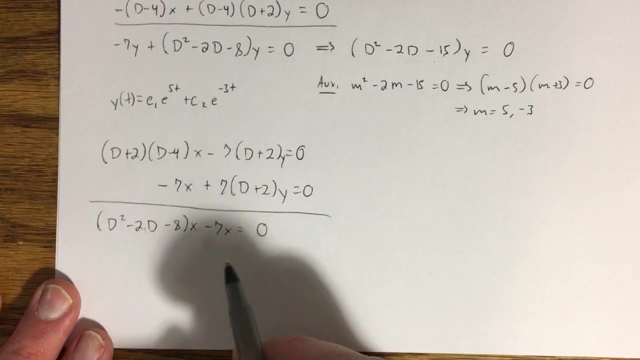 multiply things. we're going to expand these out, thinking of it similar to how we think of multiplication d squared minus 2d, minus 8x minus 7x equals 0. Notice that this is the same thing that we got in the previous case, but with an x instead of a y, So I'm expecting this thing to. 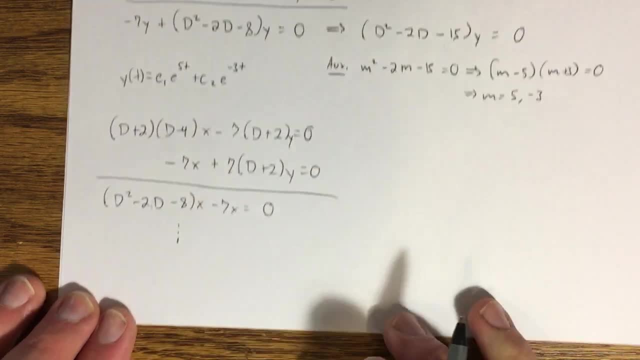 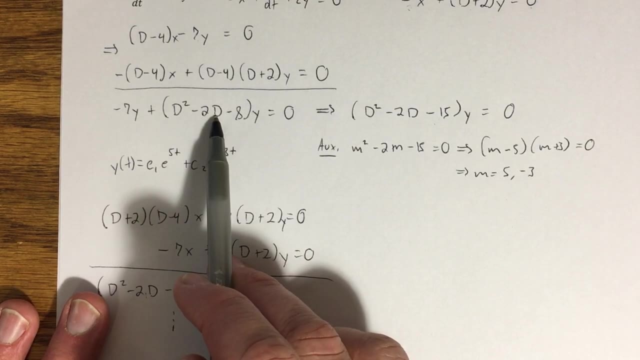 solve in a very similar way, And noticing that, noticing that this is giving me essentially an identical equation to what I have, I'm going to multiply it by 7 times d squared minus 2d, minus 7x plus 7y. Now, this is going to be the same thing that I had up here, with the only exception. 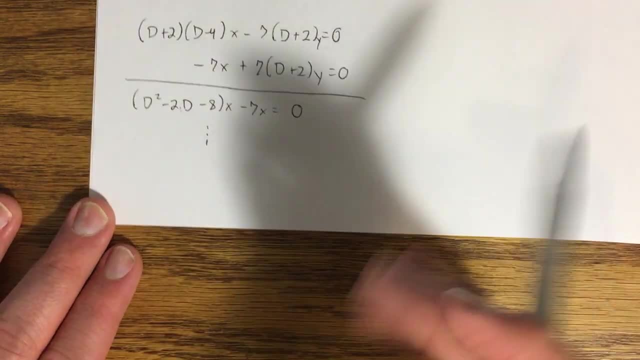 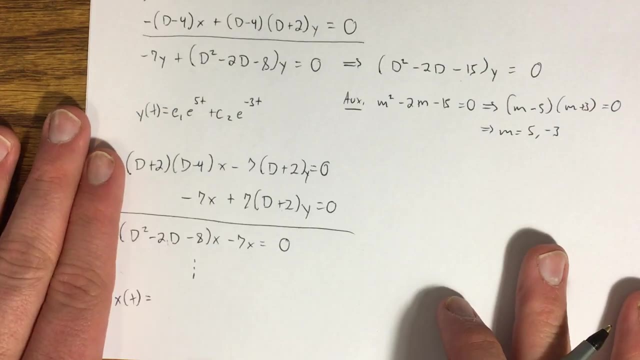 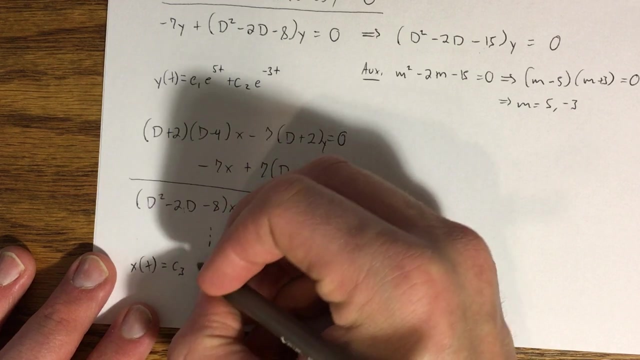 being an x in place of a y, I'm expecting my function x to have the same form as y x of t is going to look like now. one thing I'm going to be careful about is my parameters. I'm calling this c1 and that c2.. I don't want to reuse the same parameters. I'm going to call it c3. 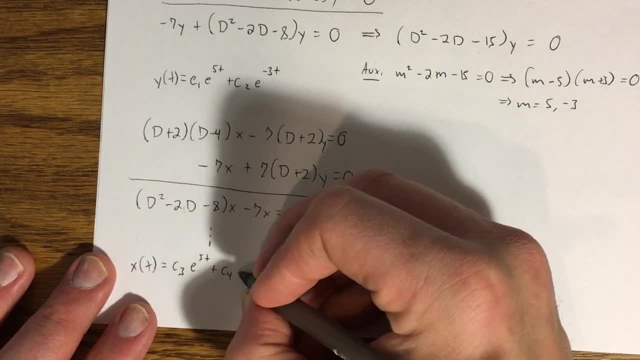 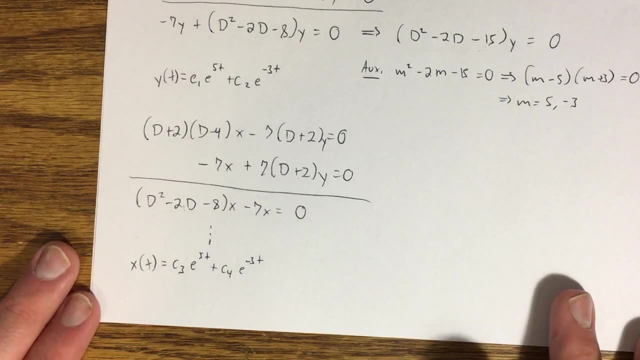 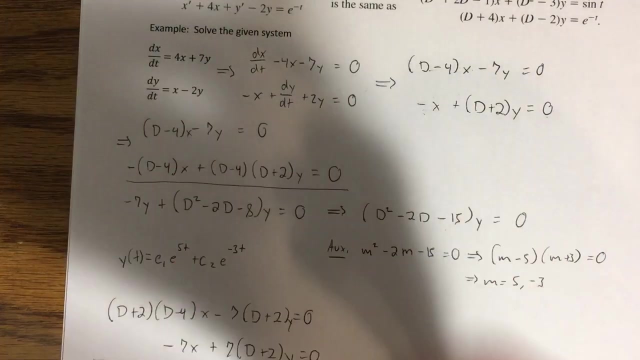 e to the 5t plus c4, e to the negative 3t. Now I have an x and I have a y. they're general solutions, but I don't. I'm actually not done yet, Because these equations up here imply that there's relationships between x and y themselves, and those relationships might 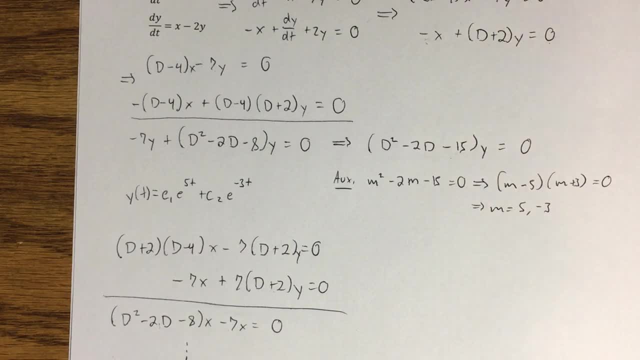 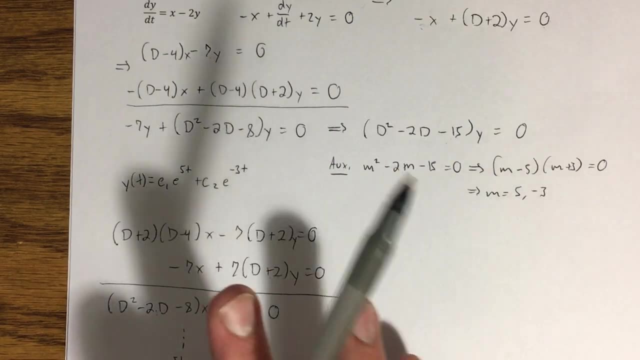 actually imply that there's relationships between the parameters we're using also. In fact, the solution to this system of equations should only have two parameters. It shouldn't have four. So we're going to try and figure out a way to deal with that somehow. 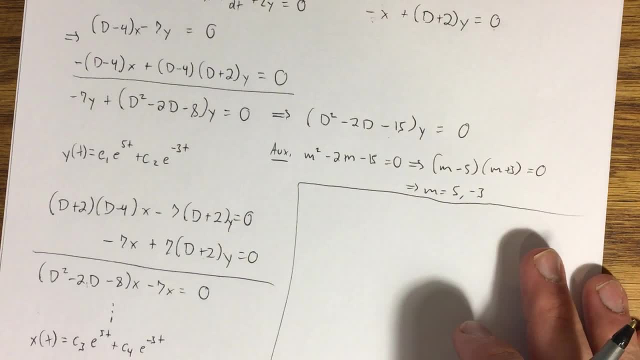 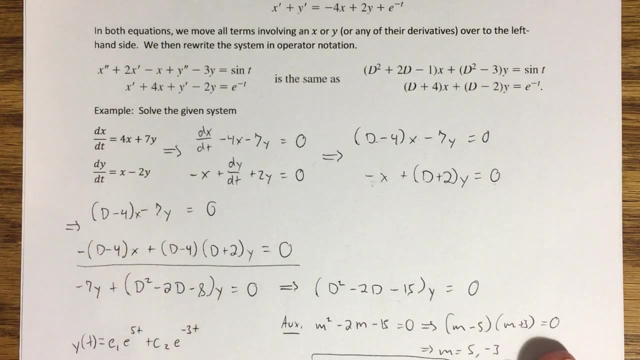 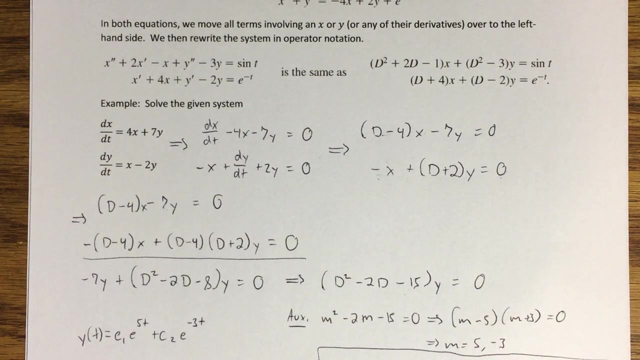 So let's, I don't know if I have enough space in here to even do this, but we'll try. What we're going to do is pick one of our two original equations up here, and we're going to substitute what we have just found into that. So if I, for example, were to do that with my 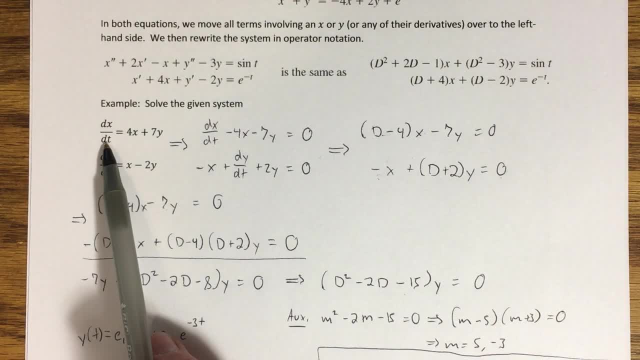 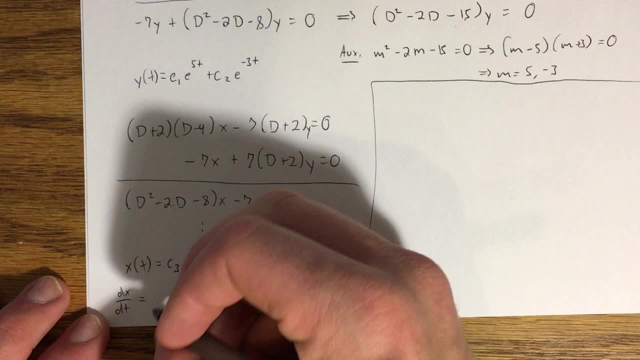 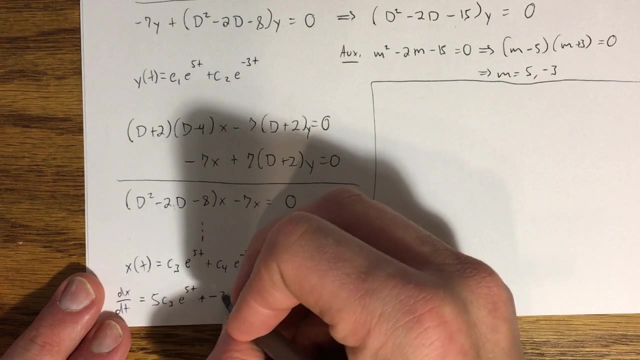 first equation I need to know what dx dt is. So I can find that here dx dt is equal to 5c3 e to the 5t minus 3c4 e to the negative 3t. Okay, that gets substituted in for the dx dt. 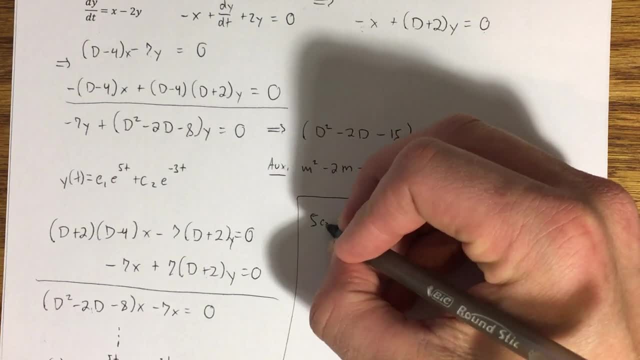 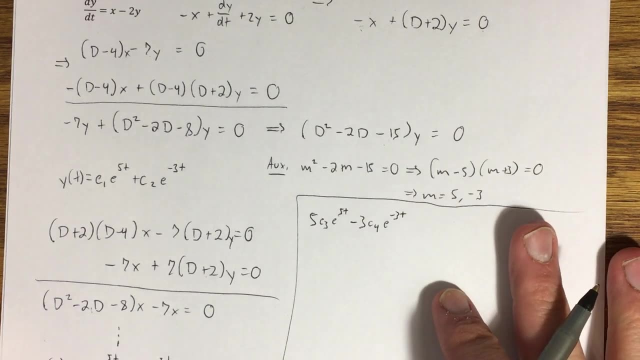 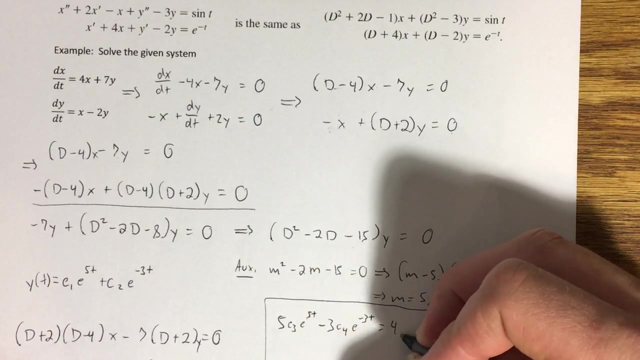 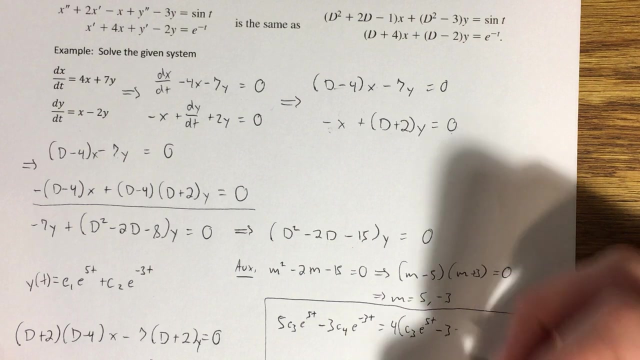 right here. So now I'm going to have 5c3 e to the 5t minus 3c4 e to the negative 3t, and that should be equal to 4x plus 7y. equals 4 times x. x was equal to c3 e to the 5t minus 3. oh no, i'm sorry, plus. i'm looking at the. 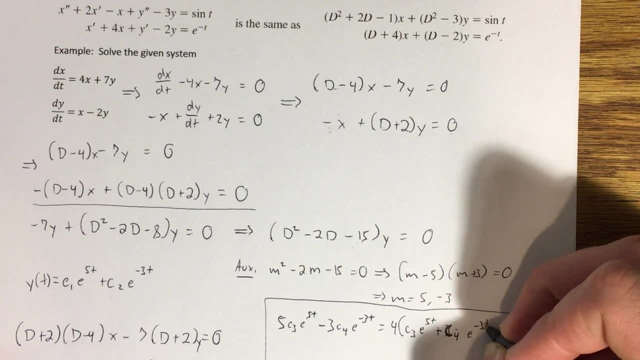 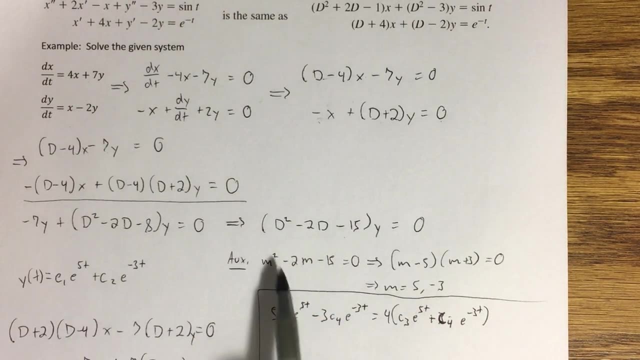 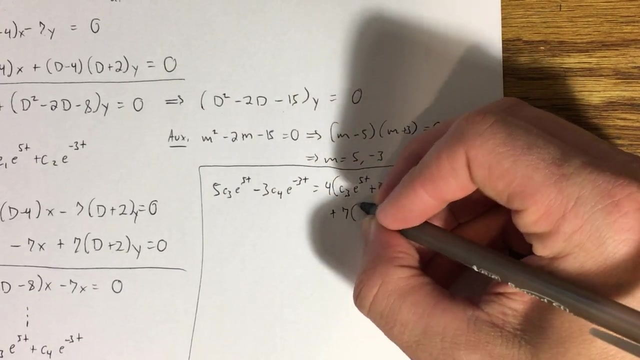 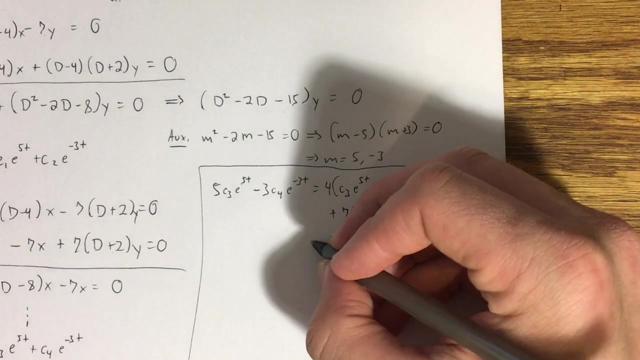 wrong part, plus c4 e to the negative 3t and y when i'm doing this, plus 7y here, y we solved for right there. so that's plus 7 times c1 e to the 5t, plus c2 e to the negative 3t. okay, let's combine. 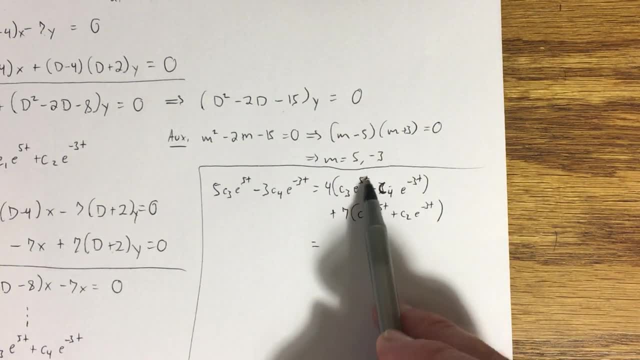 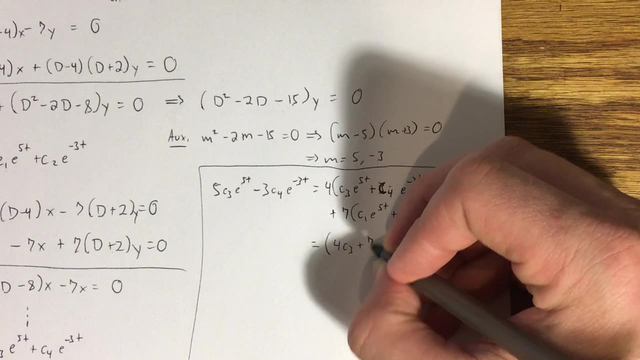 some like terms there. so if i distribute the 4 and the 7, i have e to the 5t showing up in a couple of places. that's going to give me 4 c3 plus 7 c1, e to the 5t, um, and then 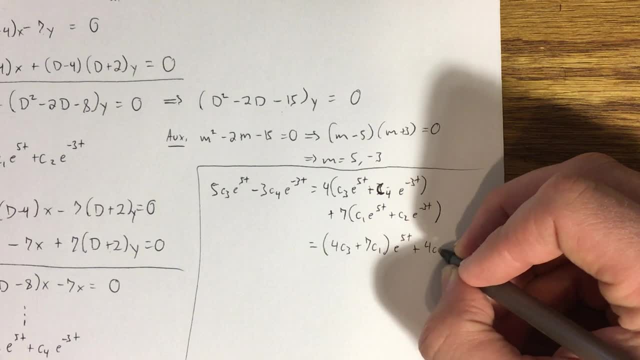 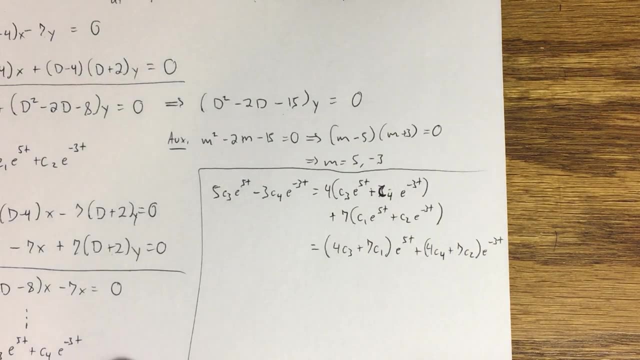 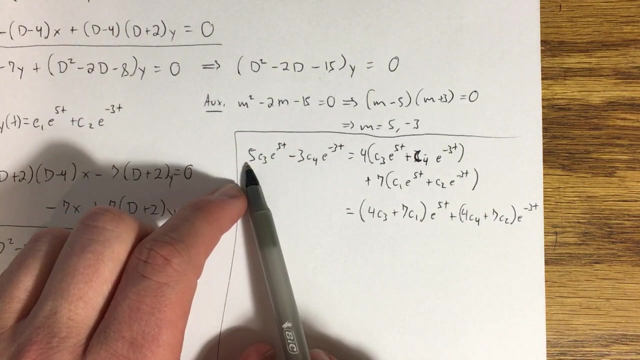 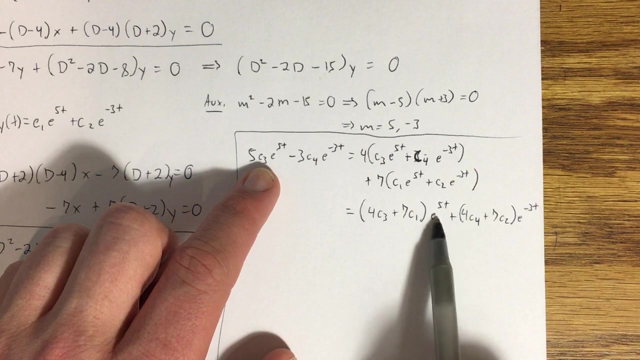 plus 4, c4 plus 7, c2, e to the negative 3t. okay, now this needs to be an identity. this side should equal this side for all values of t, which means that i can equate the coefficients on these exponential terms. so, for example, i have an e to the 5t here and an e to the 5t here, and 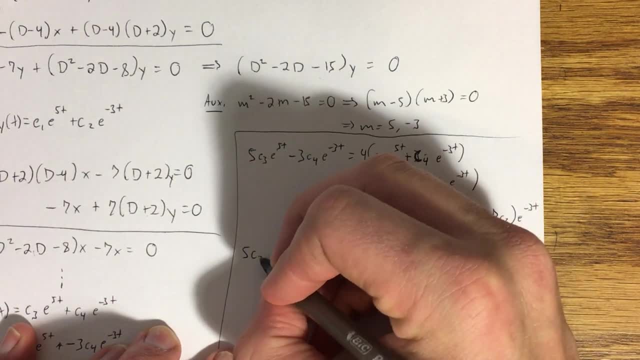 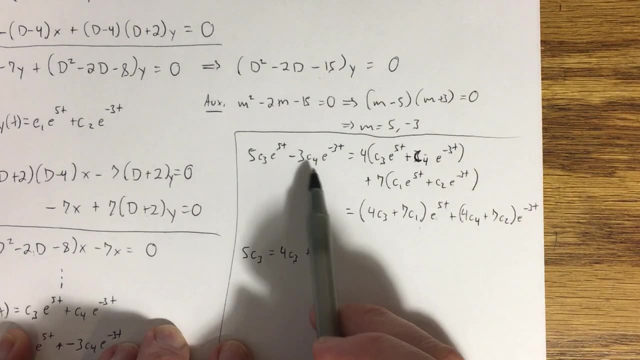 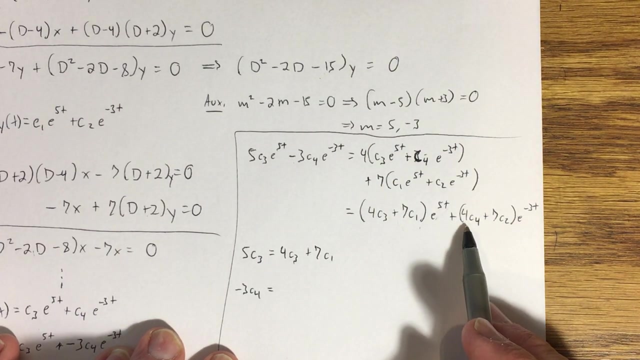 coefficients on each of those. i can set them equal to each other: 5 c3 equals 4 c3 plus 7 c1. similarly negative 3 c4 is equal to uh, 4 c4 plus 7 c2. now what i can do is i can combine some, you know, like subtract the 4 c3 over.